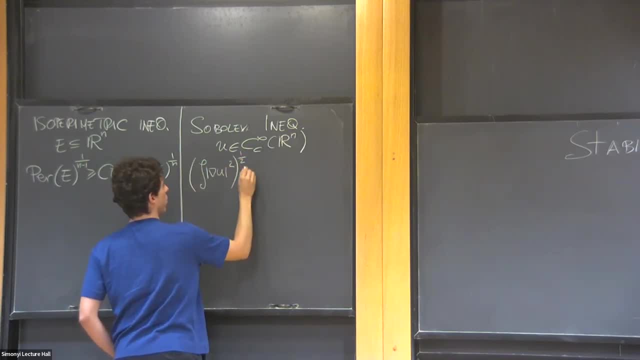 I'll talk about the L2, L2 star, Sobolev inequality, And here, instead of the volume, you have a certain mass which is the L2 star, And 2 star is the only exponent which makes sense because of homogeneities. Okay, these are very well studied. 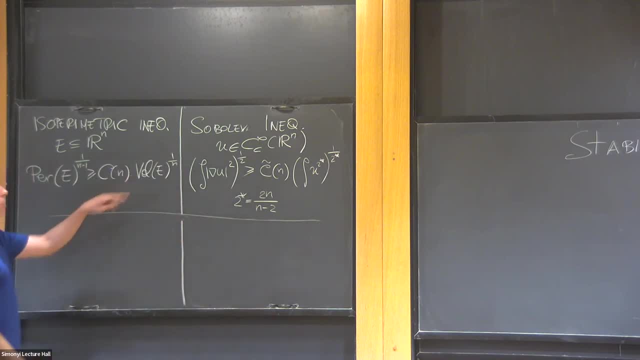 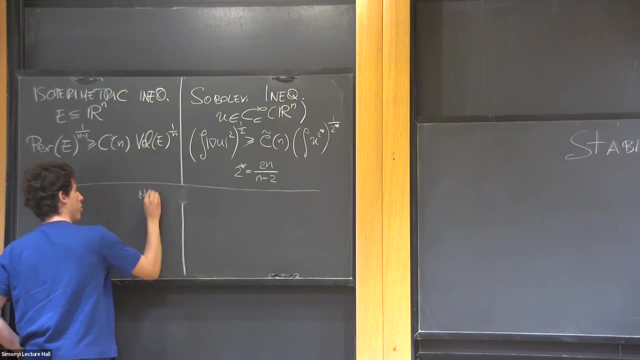 So, for example, we know the optimal constant Cn, We know the optimal sets and the optimal functions. So what are the optimal sets and optimal functions, which are called minimizers? Here they are just Euclidean bubbles, Here they are the family of Talenti bubbles. 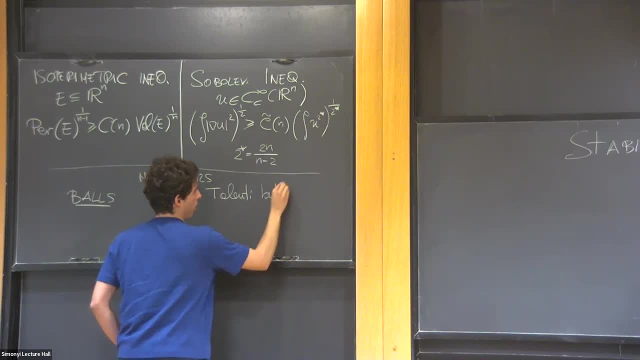 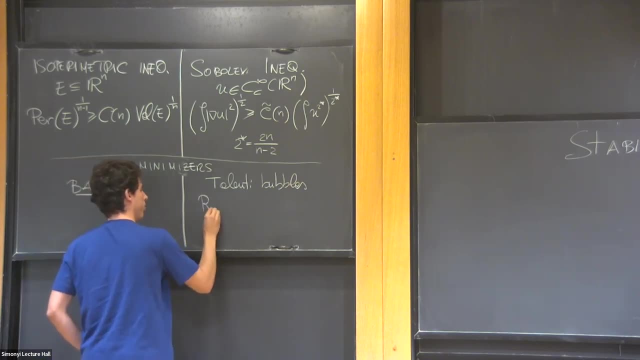 Talenti bubbles have an explicit formula, but it's not important here. What you should keep in mind is that they are radial and they are decreasing and they are not completely supported. So the profile goes something like this: Okay, then there's one last thing that I want to recall about both inequalities. 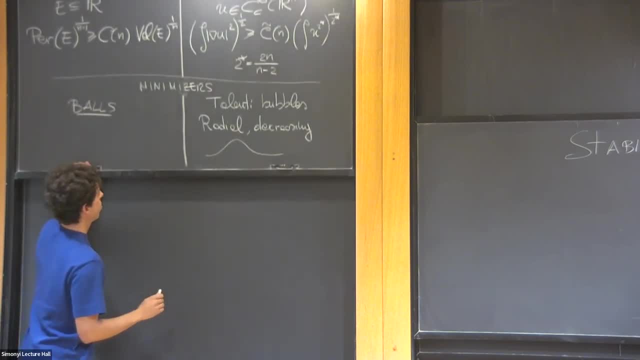 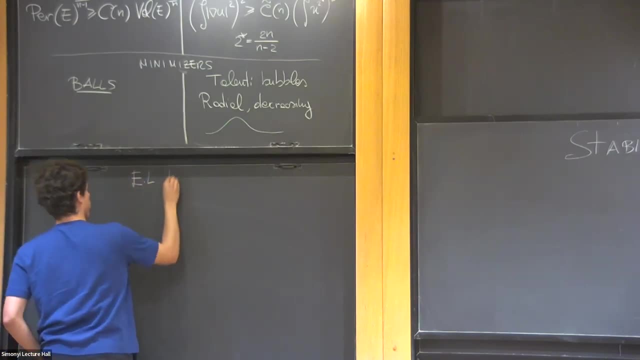 which are the L2, L2 star and the Euclidean bubbles. So the L2 star and the Euclidean bubbles, these are those inequalities which are the Euler-Lagrange equation associated. So here we have two inequalities. You can easily associate a functional to inequality, just moving everything to the same side. 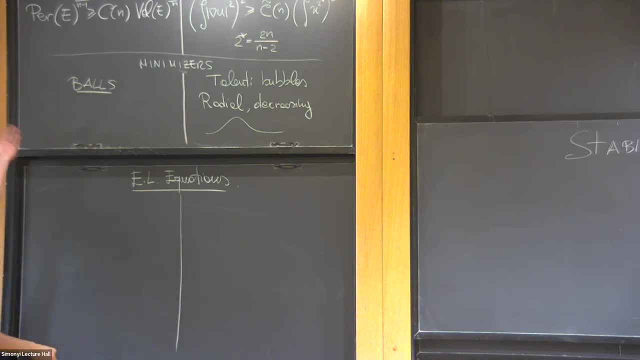 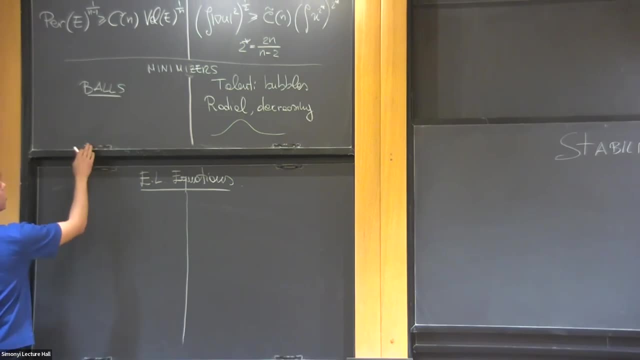 And once you have a functional and you want to study the minimizers, it makes sense to compute the derivative and this is what I call a Euler-Lagrange equation. So the stationery condition. So this is Euler-Lagrange equation. 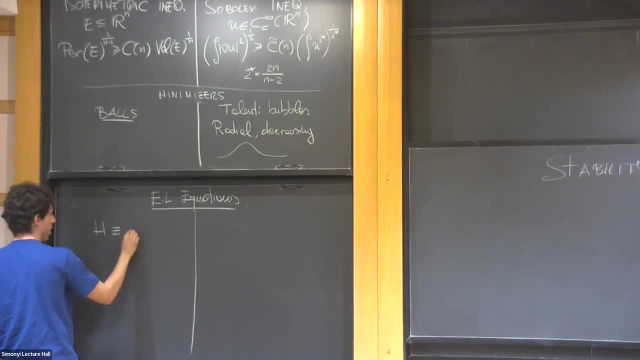 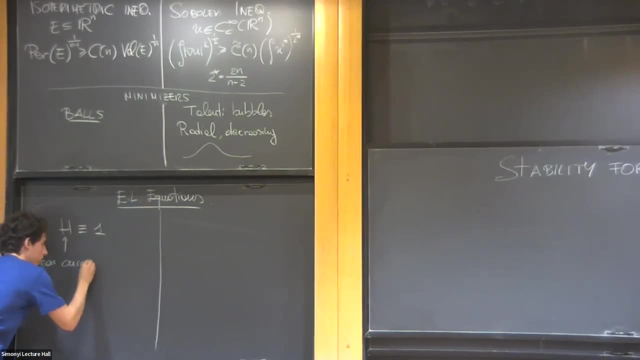 Here it's Euclidean bubbles. Here it's Euclidean bubbles h up to scaling h equal to one. This is the main curvature of the boundary. Similarly, here you get a critical elliptic equation. So I've said that the minimizers are classified. 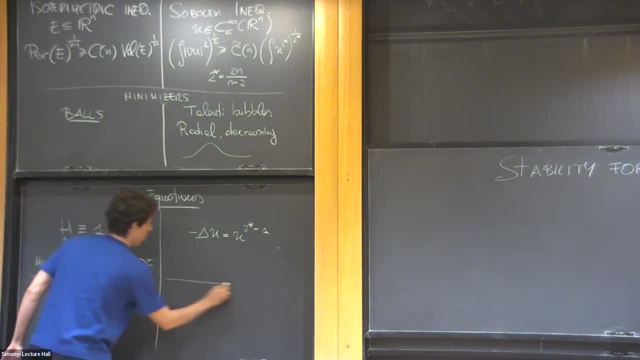 In fact even critical points are classified under some restrictions, But these are technical and I skip them. So here, once again, you get that the only solutions are walls, And here, if you restrict to positive functions, you get that the only critical points or solutions. 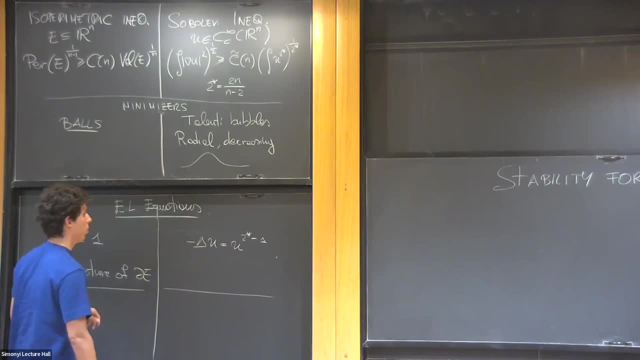 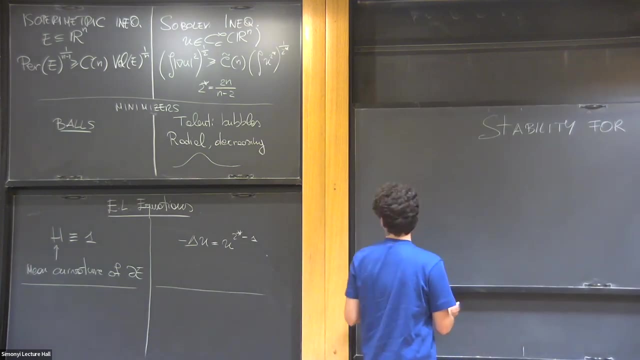 of this critical elliptic equation are talented bubbles. Okay, now I can move on and discuss what I mean with stability. Stability is the fact that if you have something which is almost a minimizer for these inequalities, you expect it to be close to a real minimizer. 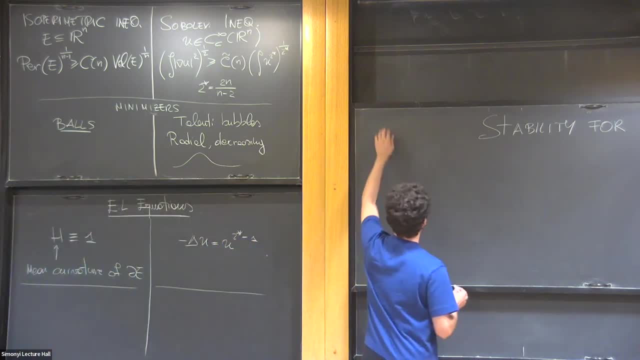 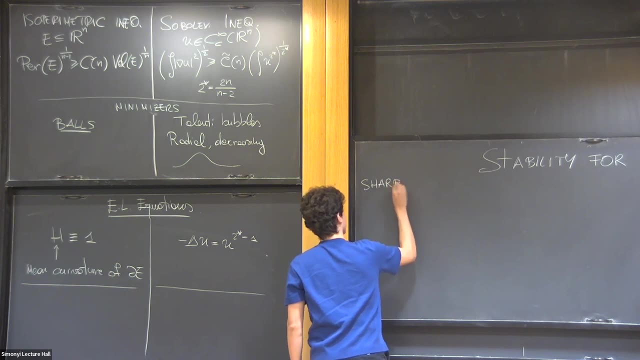 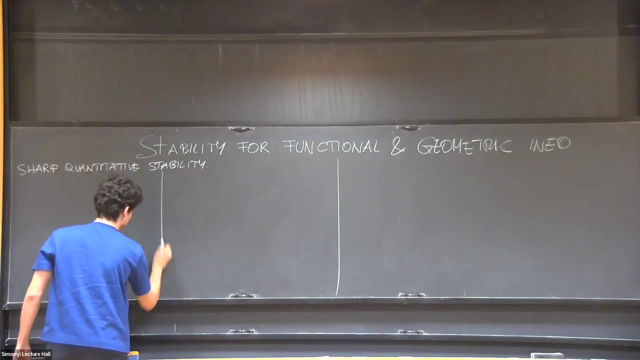 But today I'd like to discuss something a bit more specific, which is sharp quantitative stability. Instead of giving examples, I think it's best to, instead of explaining what sharp and quantitative mean in general, I give examples. I'm going to give the two examples in these two cases. 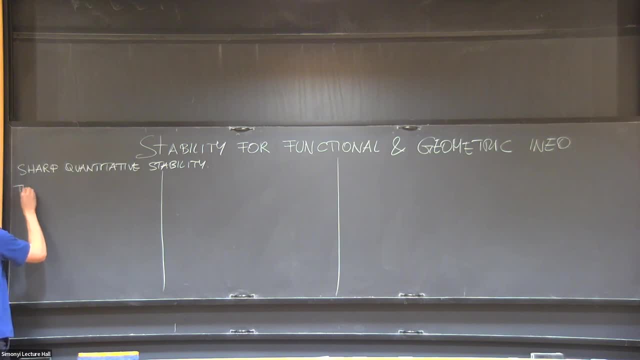 So I'll start with the statement and then I'll discuss them. So this is a celebrated theorem by Cusco Maggio and Fratelli in 2008.. And so what you want is to make the isoperimetric inequality. 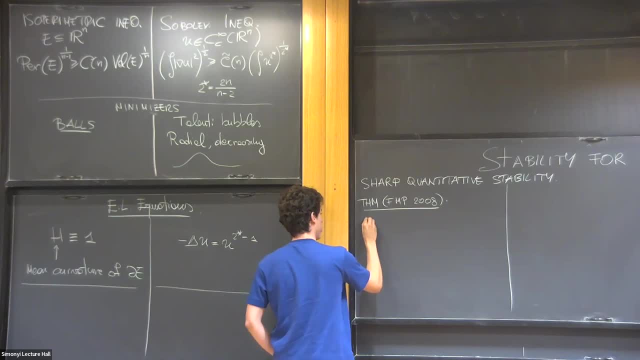 quantitative. So you take the isoperimetric ratio. The isoperimetric inequality tells you that this quantity is greater or equal than zero, But in fact you'd like to say that this quantity controls your distance from the minimizers, which are balls. 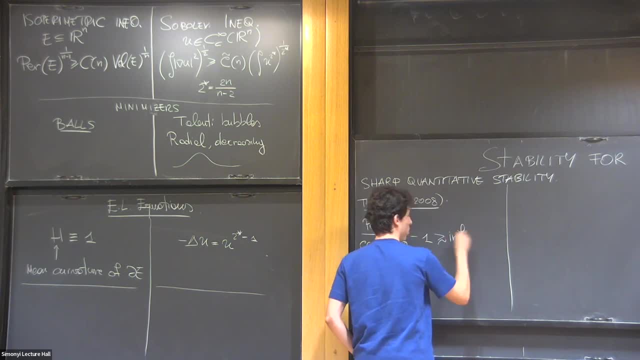 And in fact this is exactly the statement. So what I write here it's a distance from the set of balls, So you take the interval over all balls of this distance. So this is sharp in the sense that this exponent cannot be improved. 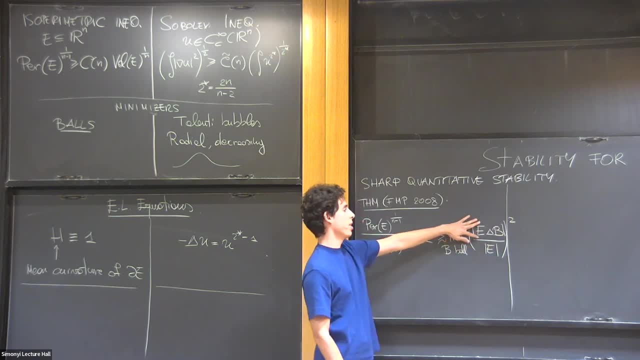 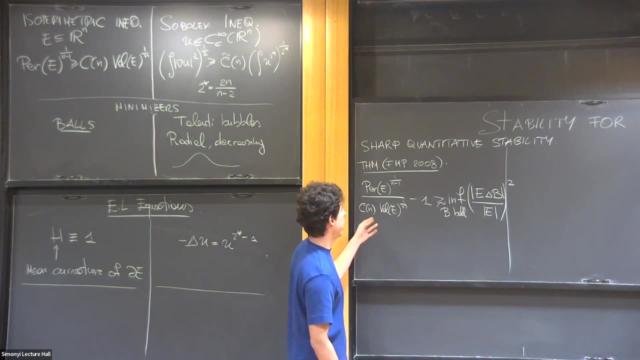 Here. this is the semantic difference. So you are taking the measure of the semantic difference And, of course, you can optimize over the ball. This was quite a breakthrough. It was open for a long time And there were partial results before with worse exponents. 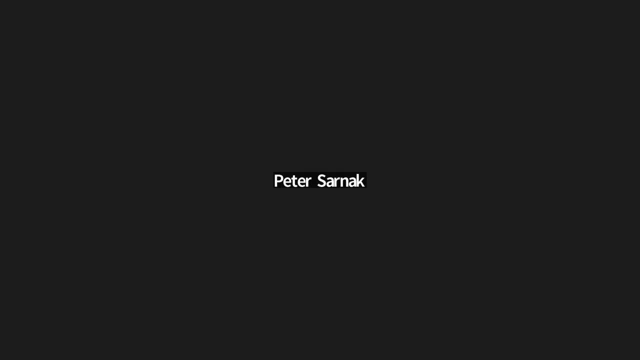 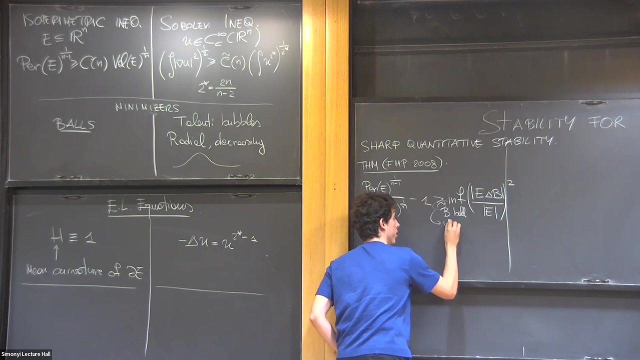 Then this was proven again In the inequality. what does the little tilde under the inequality mean? There is a universal constant here. What I've here written with CN, I should repeat it everywhere, But I'm just using the tilde. 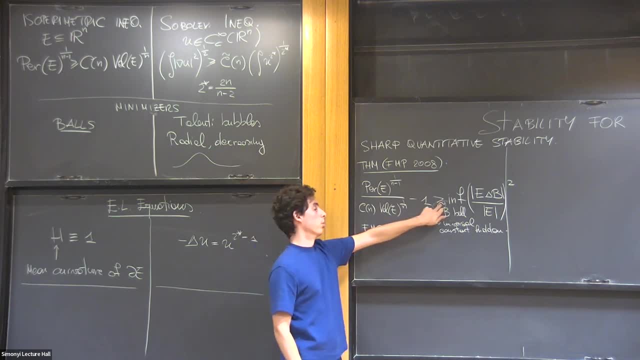 OK, this was repeated And no one is actually able to identify the constant, But that's a different topic. So the proof was repeated and a bit generalized by Figali-Maggi-Pratelli With optimal transport methods. Then it was proven again with a completely different method. 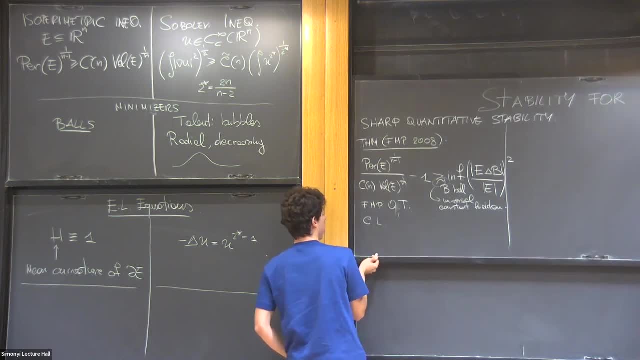 by Cicaletti and Leonardi. And then it was proven again for a much wider class of inequalities by Eleonora Cinti me, Aldo Pratelli, Fabio Rosadon and Joachim Serra. 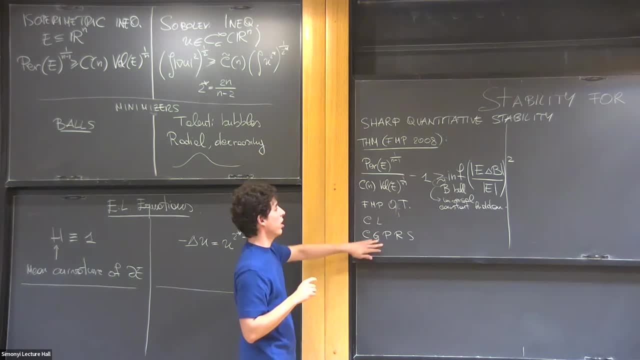 And at the very end we start from a proof of the asymmetric inequality due to Cabret, which is wonderful, And if I have time at the very end, it's one line I'd like to show it. But first, what's the situation on the other end? 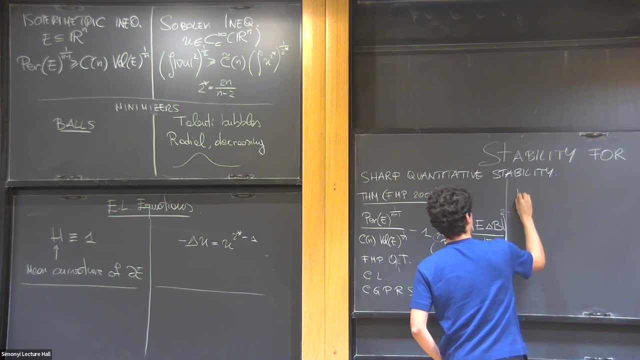 for the Sobolev inequality, We have this theorem, which is comparably easier with respect to the isoparametric inequality. This is due to Bianchi-Agnel 91. And, as you'll see, the statement is exactly what you would expect. 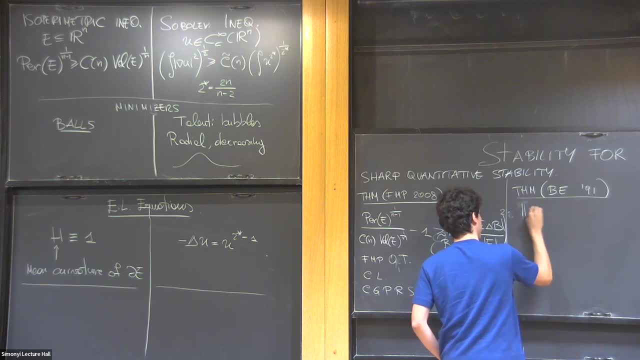 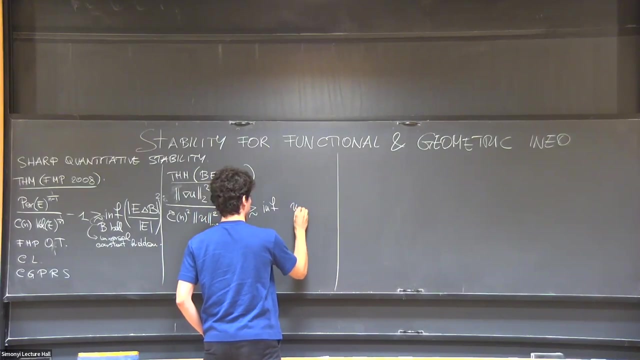 So you take the Sobolev ratio. The Sobolev inequality tells you that this is greater or equal than 0. But they're able to say that this controls the distance to talented bubbles in a very strong norm. in fact, As you see, the flavor is exactly the same. 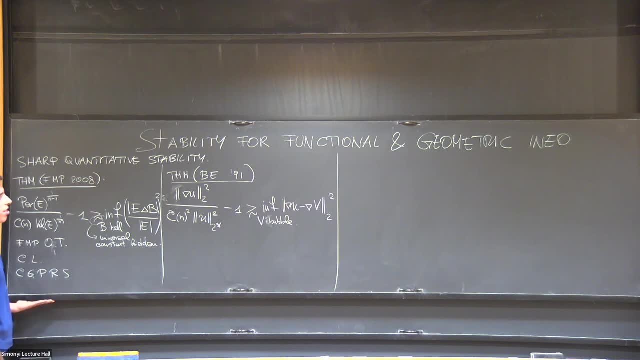 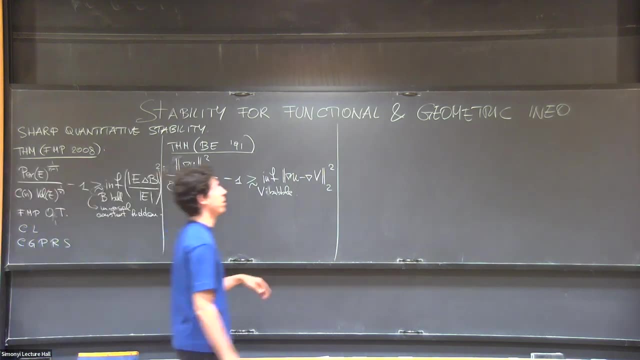 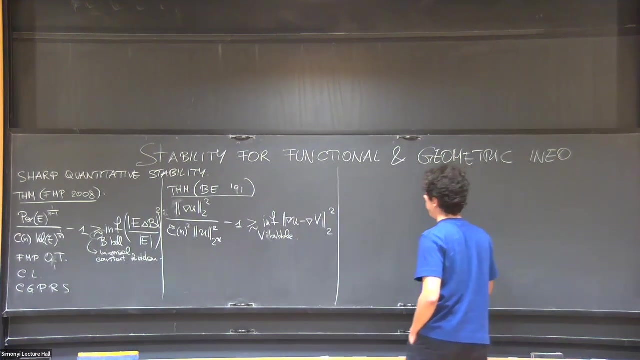 Let me mention that in some sense here the proof is by nowadays considered standard And similar methods can be applied to obtain a similar stability result for other inequalities. OK, so more or less this closes the questions for the sharp quantity stability of minimizers. 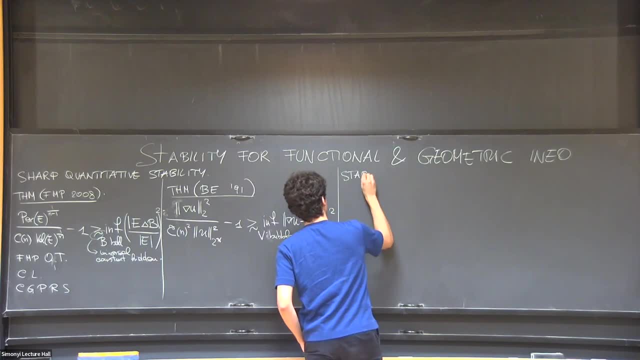 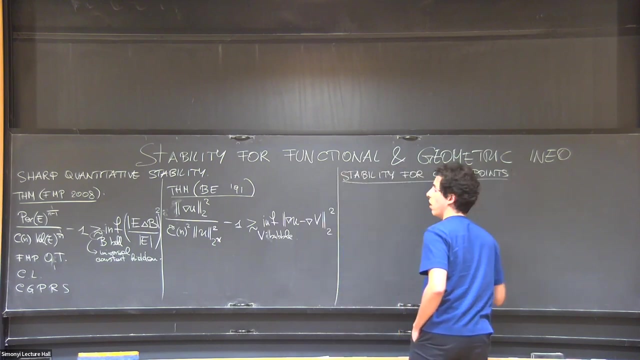 But then one can ask himself the same questions: stability for critical points. So the question here, at least qualitatively, is: if I'm almost solving the Euler-Lagrange equations, am I close to a critical point which happens to be minimizers? 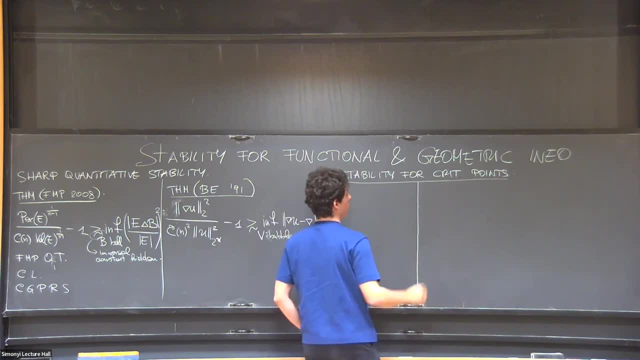 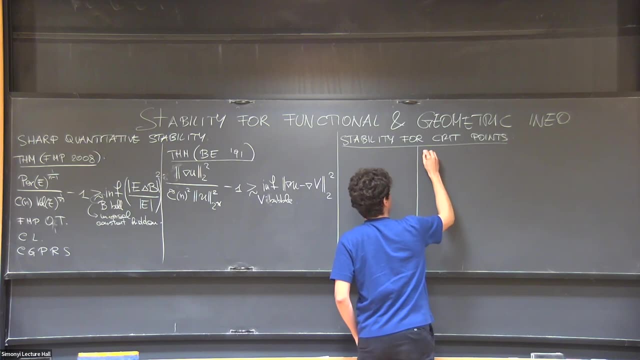 This time I leave much more space for the Sobolev case, So it will be clear why. So in the Sobolev setting one may conjecture, let's say, if I am almost a solution of the Euler-Lagrange. 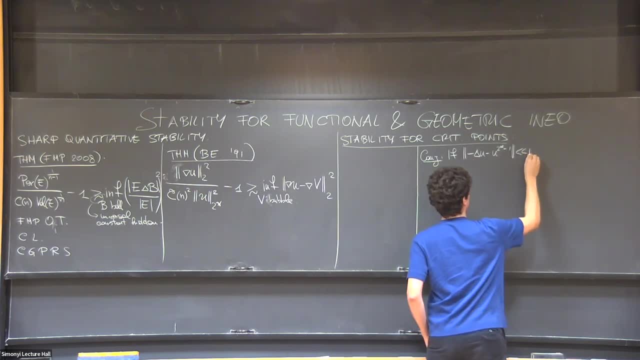 equation, which is to say that this is small, then possibly u is close to a critical point, And then the answer to this question is more or less easily: no, because just if you take two Talenti bubbles which are very distant in the space and you sum them, 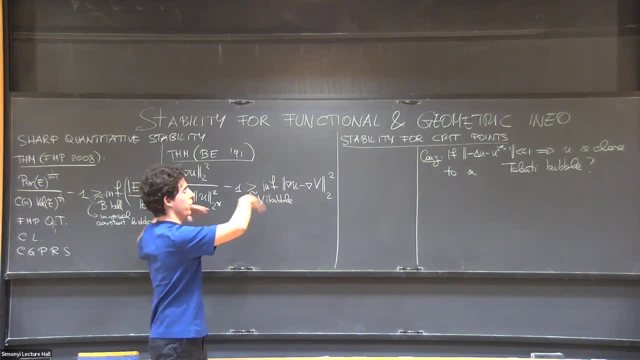 you'll get something which satisfies this, But of course, it's not close to a Talenti bubble, Sorry, Yes, please, Don't you have to stick to positive solutions? Yes, I do have. This is something that, here, I have completely omitted. 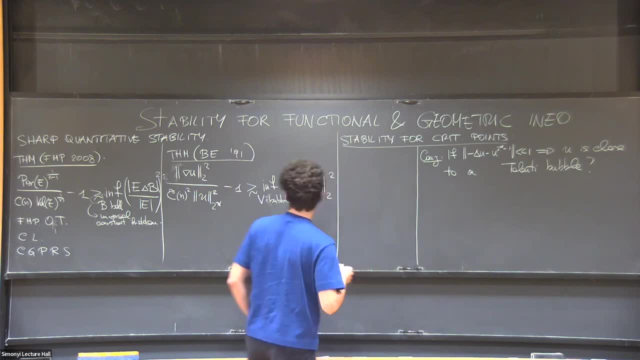 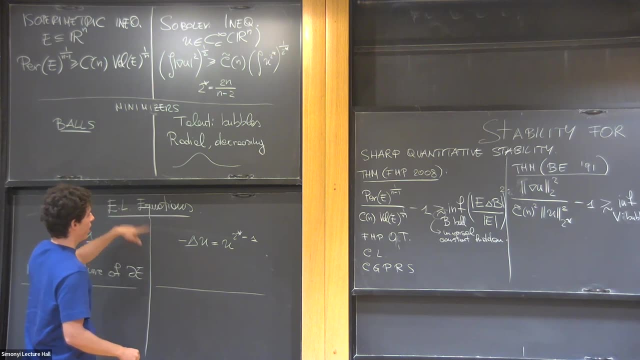 But you can see that the solution is not close to a Talenti bubble. So this is a positive solution. But more or less everywhere, like here, I'm saying that one can really say just easily that the only solutions of these are Talenti bubbles. 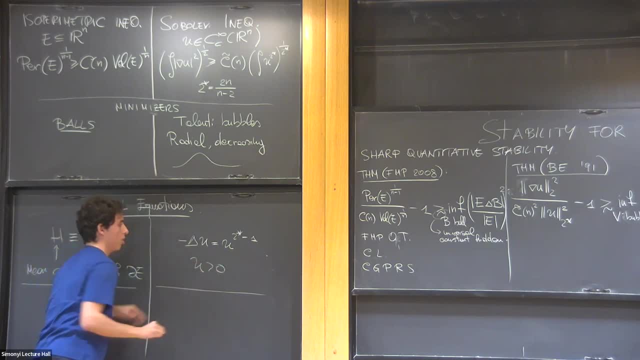 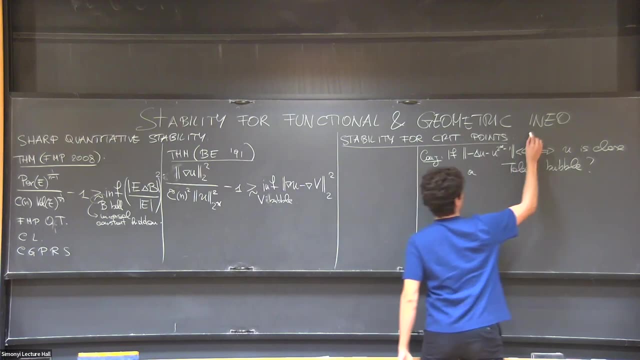 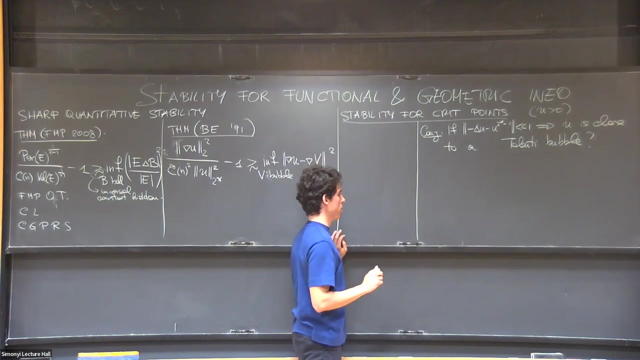 but this is false, Like there are sign-changing solutions, There are infinitely many Not very well studied on this Exactly, yes, More or less everywhere. But in some sense, studying the Sobolev inequality, it's rather natural to restrict to positive functions. 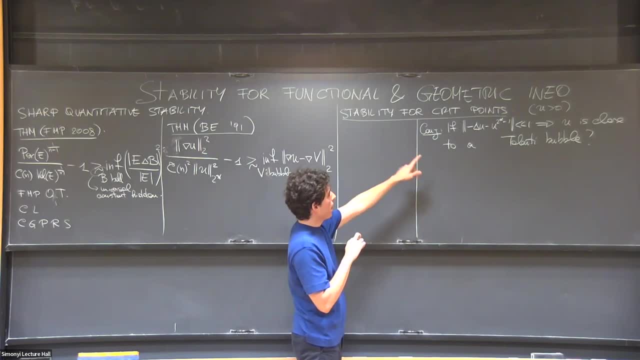 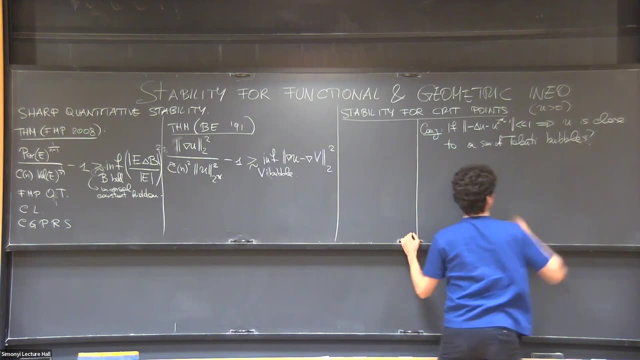 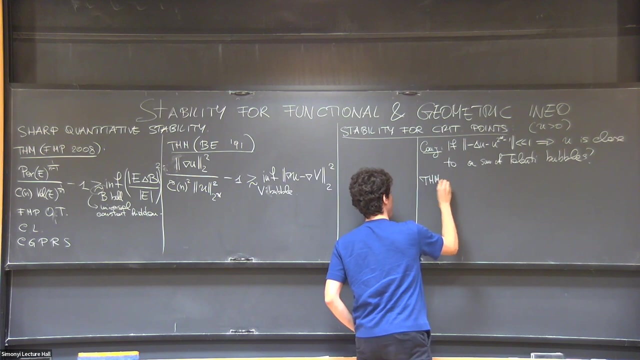 Anyway, I think it. Thank you. So this is false, But maybe one can guess. maybe to a sum of Talenti bubbles This could be true, at least more true than before, And this was made a theorem qualitatively by Struve in 1984.. 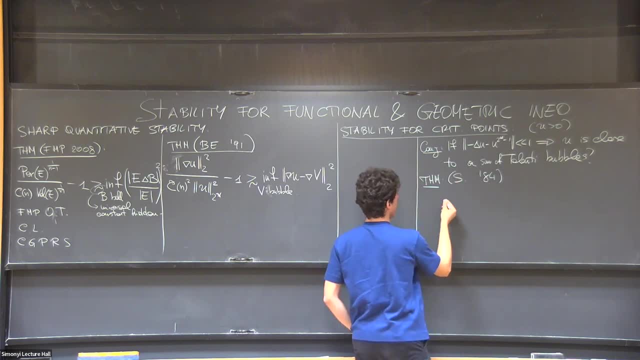 And what's the statement of this theorem? Once again, the statement is very natural. There are some technical conditions, I will skip. One of them is the positivity, And what you get is that If this quantity, and here the natural norm- 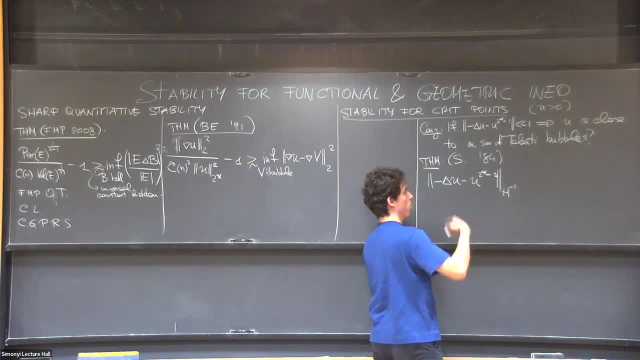 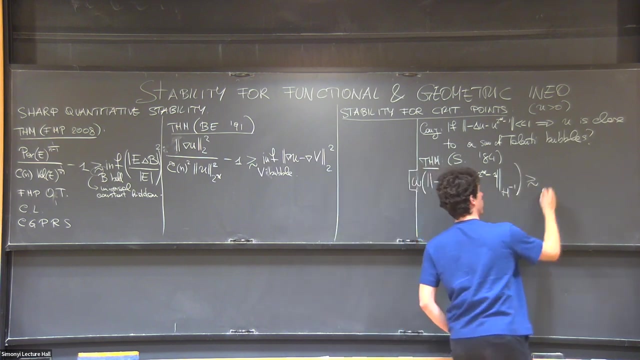 to consider is h minus 1, because you are taking the norm of a differential. If this is small, non-quantitatively so, here you have to put a modulus of continuity. then this controls the distance between u and the sum of Talenti bubbles s sum of Talenti bubbles. 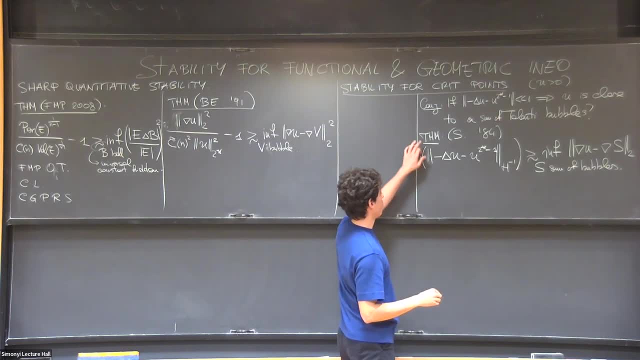 And this is purely qualitative, obtained by compactness, And before getting to something quantitative, we need to wait a bit, And the quantitative version was done by me and Alessio, And more or less, but only in low dimension. If the dimension is between 3 and 5, then we can remove omega. 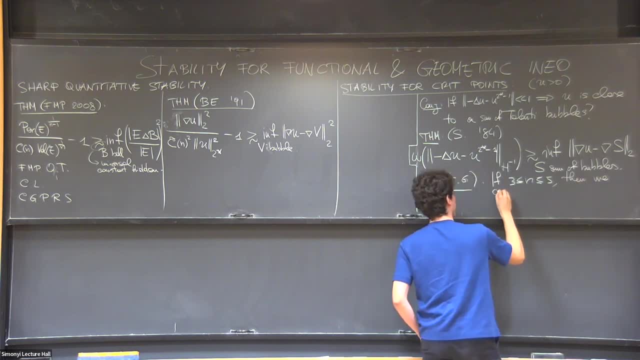 And the result is sharp. We just removed omega and this is sharp. You cannot put exponents anywhere. it will become false. But this is only in dimension between 3 and 5, and in the paper, in fact, we proved that. 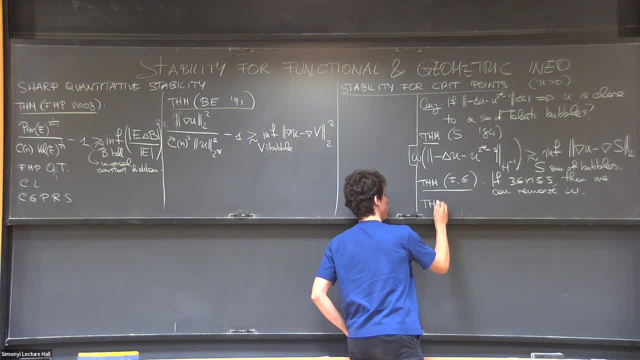 it's false. in higher dimensions, dimension, Get something. in another dimension, we have to wait for Deng-Sun and Vibe. I don't know if I think it's still up in print, but in dimension greater or equal than six, let's. 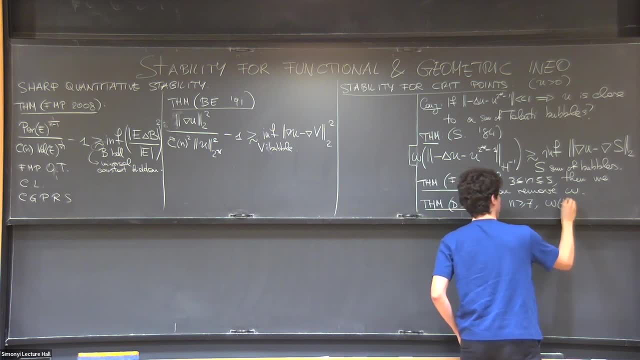 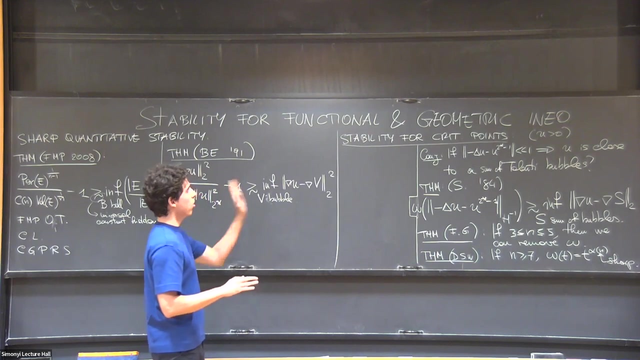 say seven, then one can put omega equal to t to alpha n and they can identify the sharp exponent. And for dimension equal to six, there are logarithms appearing, but they are able to detect them. Okay, so in some sense also the sharp stability, the sharp quantity. 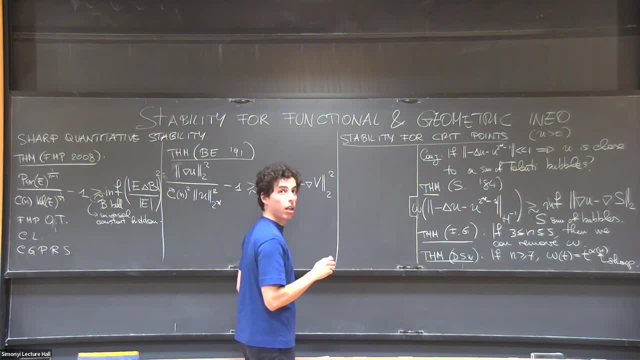 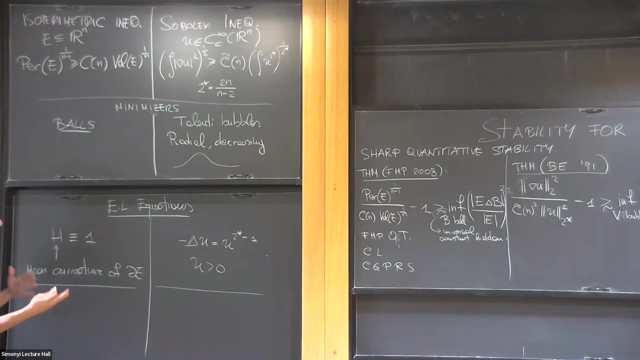 stability for critical points is closed. for the Sobolev inequality, It remains just to wonder: the only missing piece. is the same result for the isoperimetric inequality? That is to say, if something almost solved this in a reasonable sense, then it's close to? 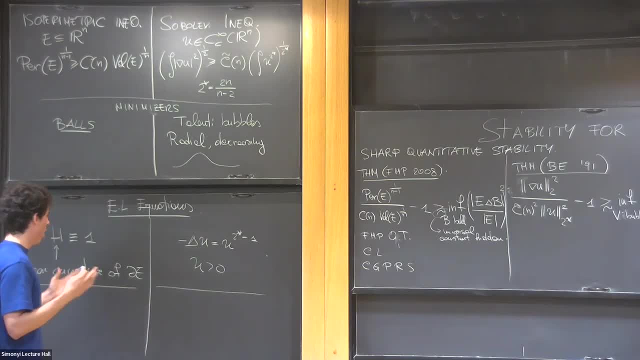 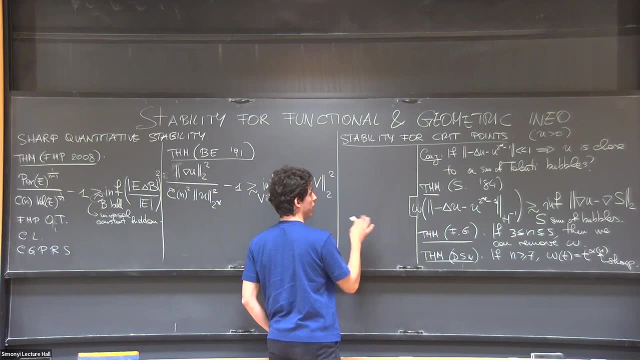 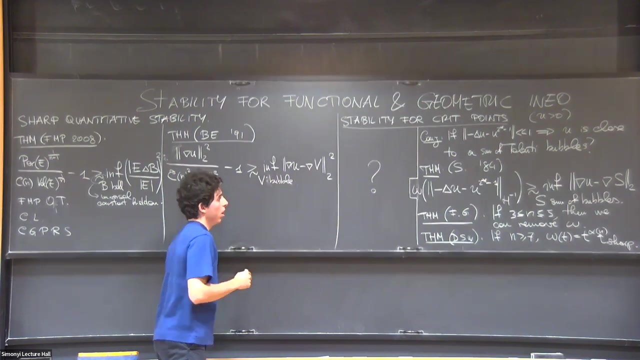 a ball. This would be false, Close to a collection of balls Qualitatively. we know this, but there is no sharp quantitative result in the correct norms. So here this is in some sense the only missing piece of the puzzle. Yeah, Okay, And I'd like to use literally the last. 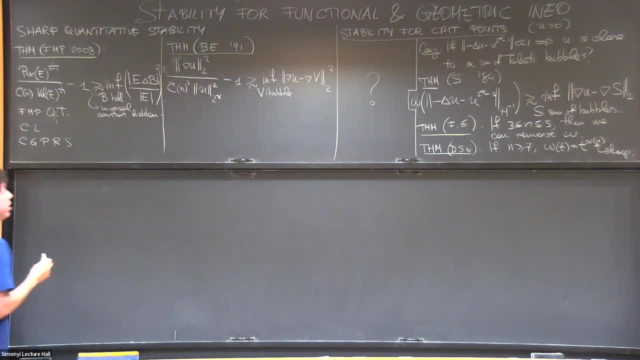 two minutes to show something which is not mine. This is a one-line proof. there's a superimetric inequality due to Cabrin. This is what we used in this work here. In this work here, we proved the stability for a wide range of isoperimetric 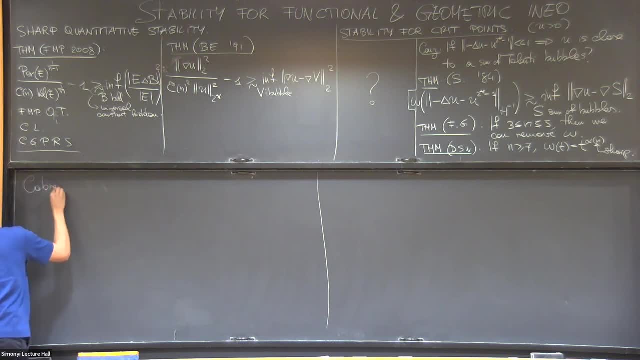 inequalities. But that's not why I want to show it to you. I wanted to show it to you because it's wonderful And it was used recently by Simon Brandel to prove an isoperimetric inequality in codimension one And, as you'll see, the proof can be- can be given in the last two minutes of our talk. 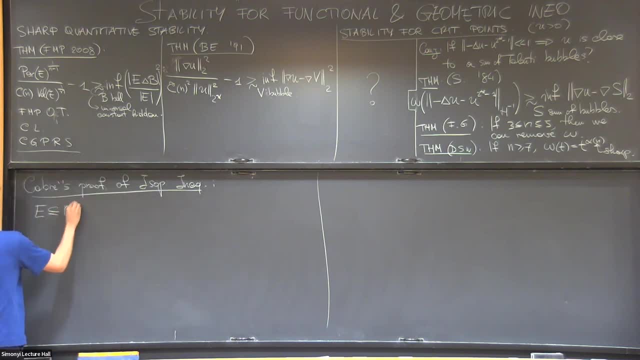 So you take a set E And normalizing you may assume that the volume is equal to the perimeter. It is easy to obtain And therefore this guarantees that you can solve the following system. This is analysis two. Okay, Then just using the boundary conditions, one obtains that the gradient of view takes. 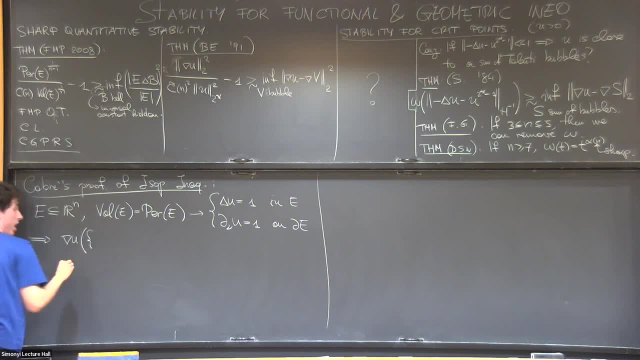 a lot of values. The precise statement which is elementary- to prove this is an easy exercise- Is that even if you restrict to the points where the action is positive, you still get the whole, the whole unit. So the whole unit ball is contained in the image of the gradient. 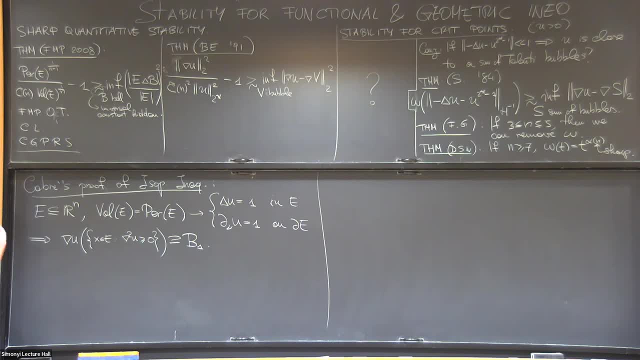 And now if? if you have seen the proof through optimal transport or through the- not a map- of the isoperimetric inequality, you can expect what is happening. Thanks to this, you can do A change of variable and writing down the Jacobian. 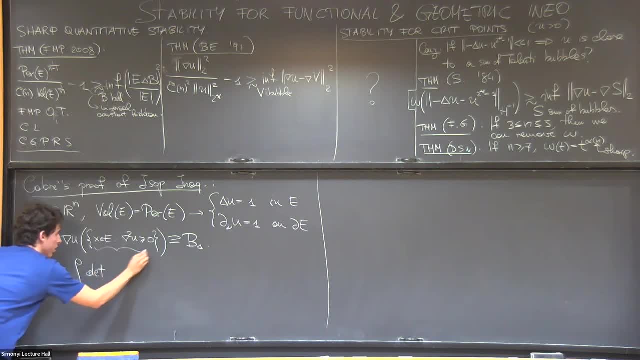 You will get that the integral over this set that are the tilde of the Jacobian, must estimate be one. But then you know you have a determinant, You have a condition on the Laplacian. It's very natural to estimate these using like. 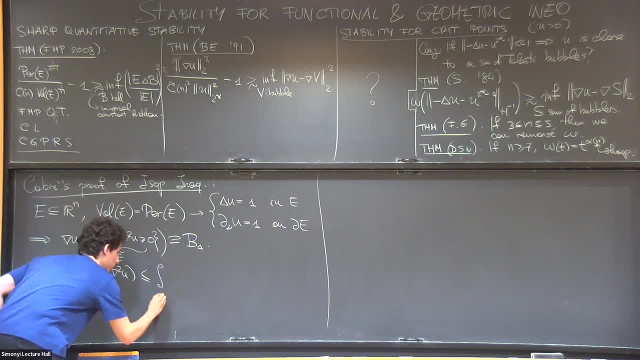 the inequality between. are you making mean and geometric mean, and you get Laplacian divided by n to the power n. Here You just replace E tilde with E. Here you replace Laplacian with one, because you know it, and you end up with this. 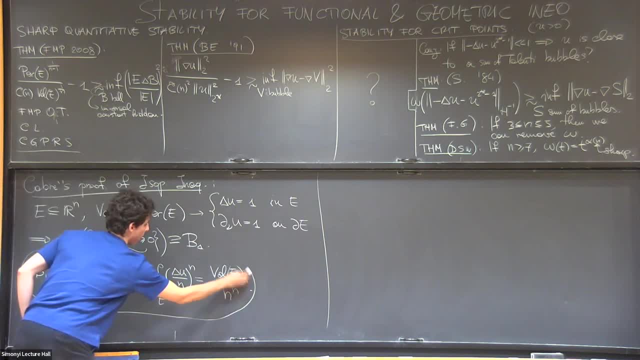 And it turns out that this is exactly a superimetric inequality. Like under this constraint, This is equivalent to a superimetric inequality, which is rather magical if you don't believe it, because there are some numerology. There's some numerology going on. 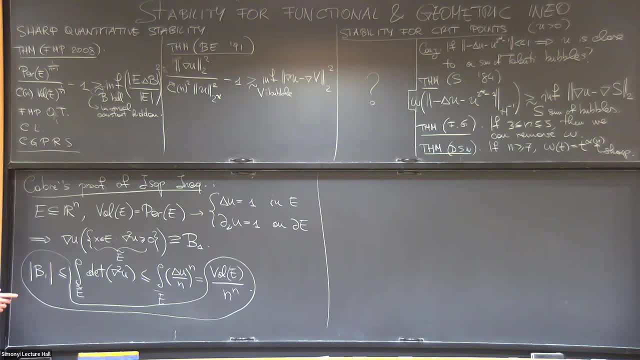 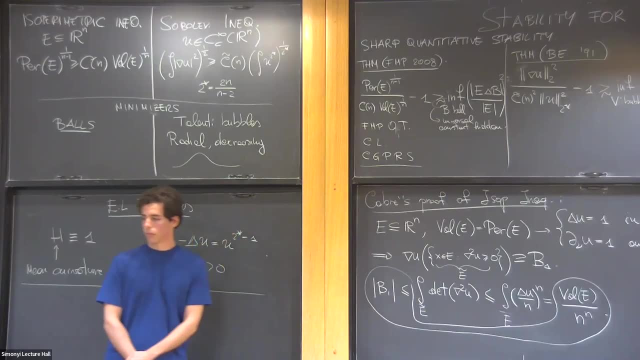 You can notice that everything is on identity for the balls. So this must be the superimetric inequality. and with this I would conclude. Thank you very much. In which way do you actually measure to do? Would you like to measure somehow, say, if you have to shoot a conjecture here on the 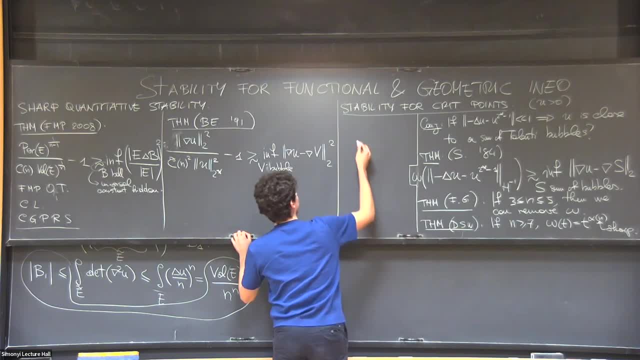 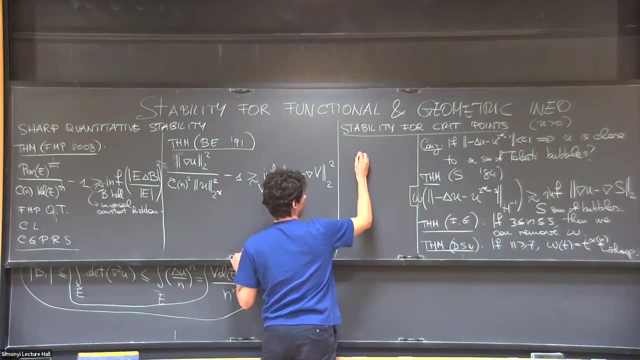 How do you want to measure being far from the oscillation, I mean age, and how would you measure the oscillation? Well, the oscillation kind of looks natural, but age Like something like this would be amazing, Using this in L2 or I mean. or there is in some sense the easy result, but maybe less interesting and it's less clear if there would be a sharp quantitative version which makes sense a lot. 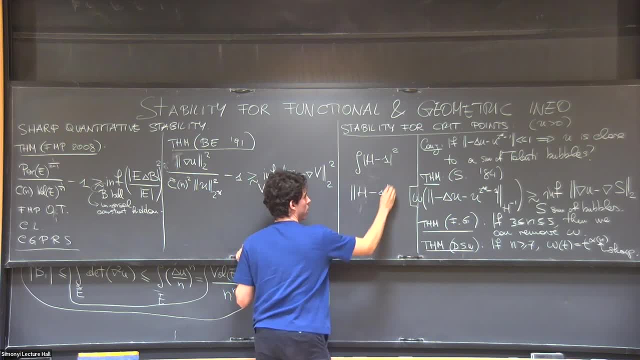 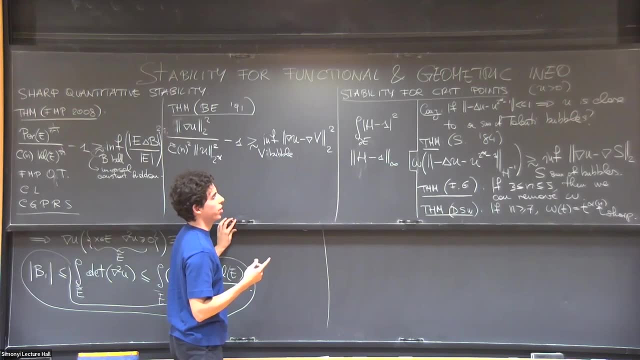 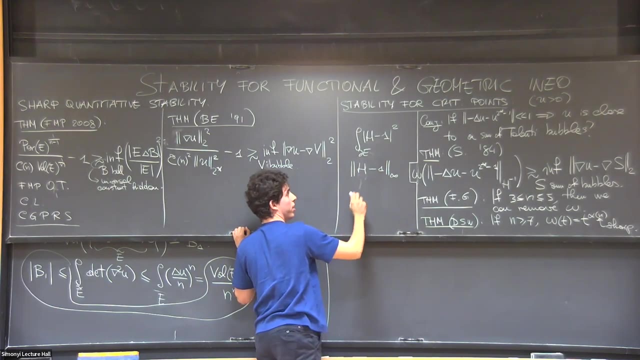 It's something like this: here you write down the number and, on the other hand, one should really take care of what kind of result it wants to obtain, because I mean, in fact, that one would have two different results, Like, if you assume something like this, then you would expect to get tangent a collection. 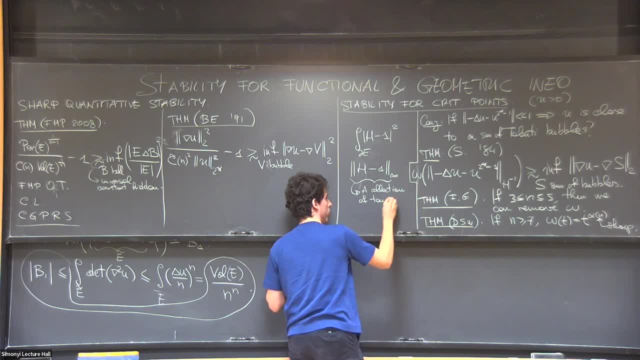 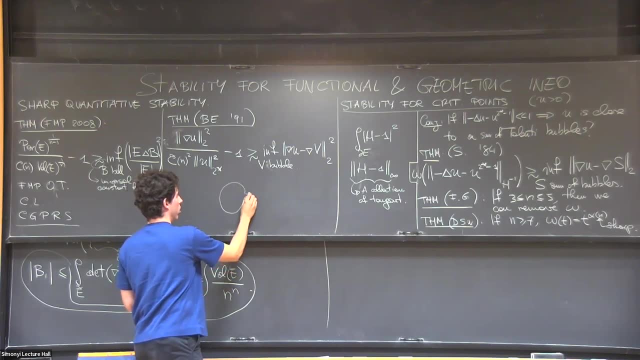 of tangent balls, Because it turns out that one can in fact produce two tangent balls Keeping the main curvature close to one. on the other hand, here you can even produce stuff. You can even produce stuff like this and many of these. So here are tangent and here non-tangent. 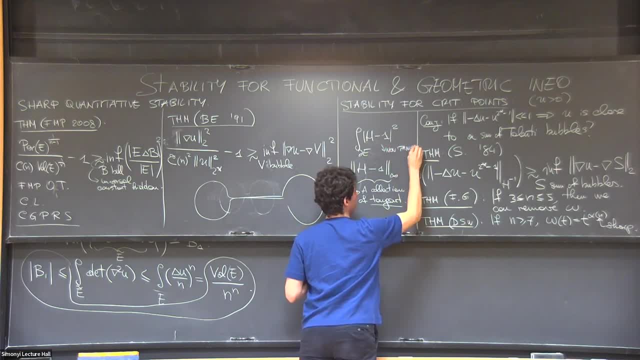 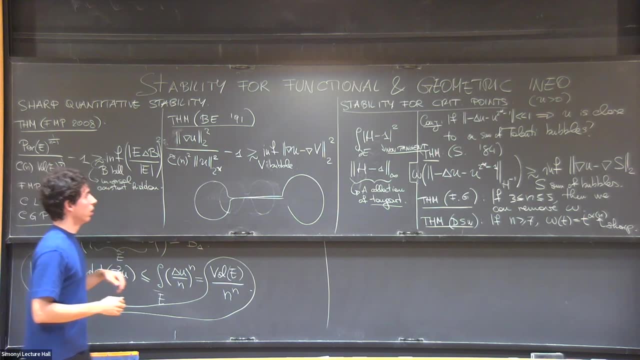 And you want to measure the symmetric difference of the set? Possibly, Yeah, These guys Correct, You cannot really open something much better, like at the level of the perimeter, Sure, But what is known is that with this norm- okay, here I might say something false, but with this norm it's known qualitatively. and with this norm is known quantitatively, but it's non-sharp. 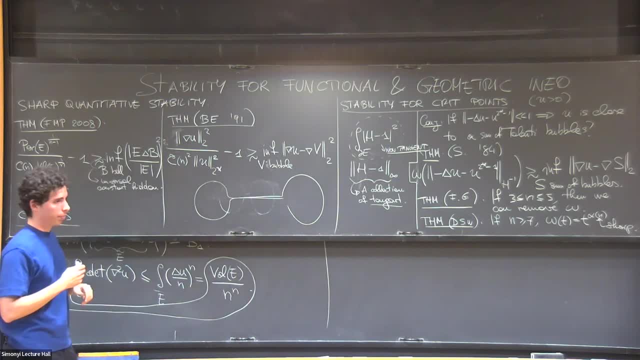 Like no one believes that this point is sharp. It's just around this point. Qualitatively, you mean, if there is global, if the set is small, you're close to a configuration like that. Indeed, And always, there is always some kind of estimate on the volume. 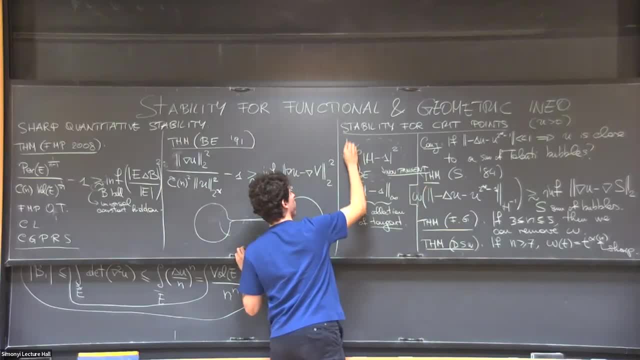 Like here. I'm dropping some assumptions going on, but here you'd have two Totally Indeed, I don't know, 25 V1. And here one absolutely the same. Like you have to still keep the energy bounded. 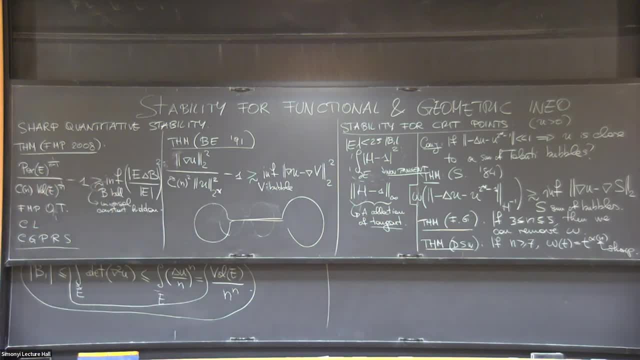 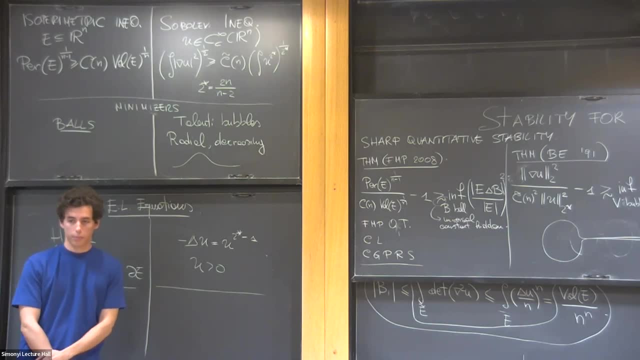 Yes, Any questions? This is kind of an off-the-wall question. I've always worked in higher dimensions, So recently I've started thinking about dimension two And you have all this nice machinery. Can you ever, if you ever, find any problems, a problem in dimension two that you can solve using it? 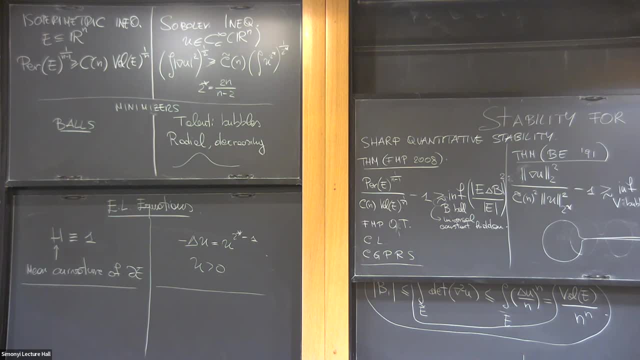 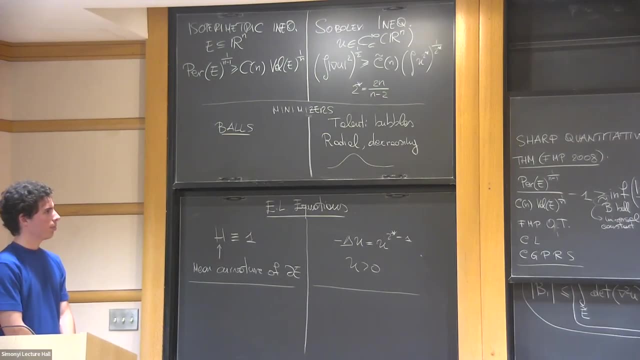 Not that I can think of Like the main issue, like whatever concerns the Sobolivian equality. at least L2, L2 star really breaks down in dimension two. Yeah, And I actually don't think that there's really anything in dimension two. four: 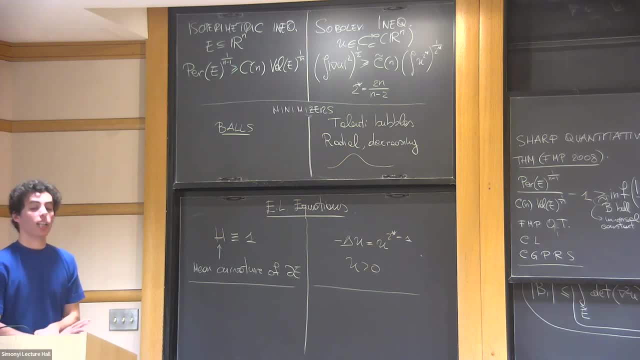 I don't want to say something false, But the answer is sadly, no. Oh, it's too bad. Yeah, We have all this good machinery. Well, but if you assume H minus one in L, infinity in two dimensions, that's like saying that's so strong, right? 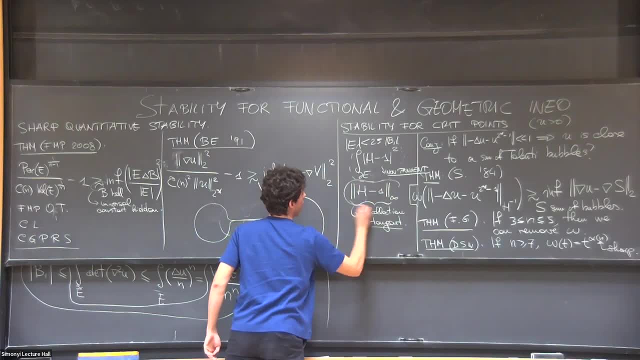 I mean essentially the curve. Oh, you mean this. Yeah, I mean, then maybe it's doable, I don't know, I don't know if Ah, no, Yeah, In two dimensions that is much, much stronger. 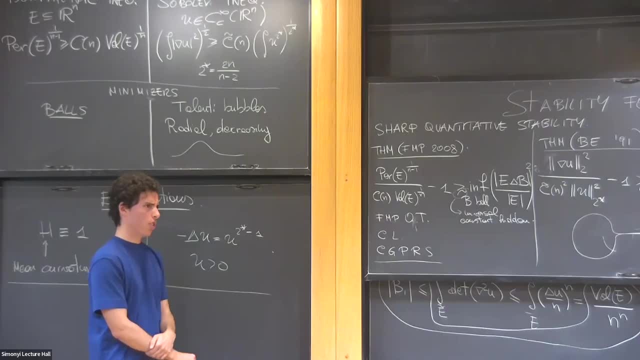 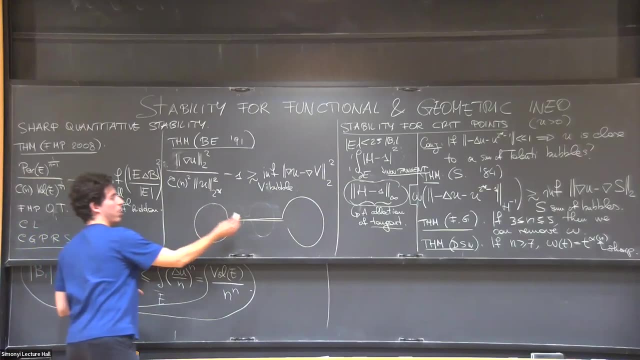 Yes, In two dimensions. I think that you can not even have two tangent bolts Exactly Indeed, Yeah, But I guess this becomes like more or less elementary in two dimensions. Yeah, Yeah, Because everything is one dimensional here. It's more or less a second derivative. 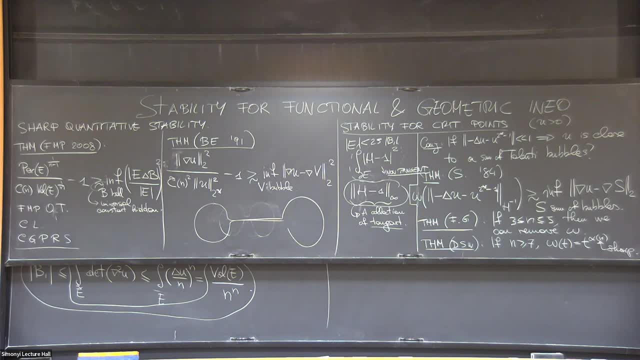 I think you are accurate. Yeah, Yeah, Yeah. Well, that's more or less correct. what would happen? Okay, So let's thank you again. 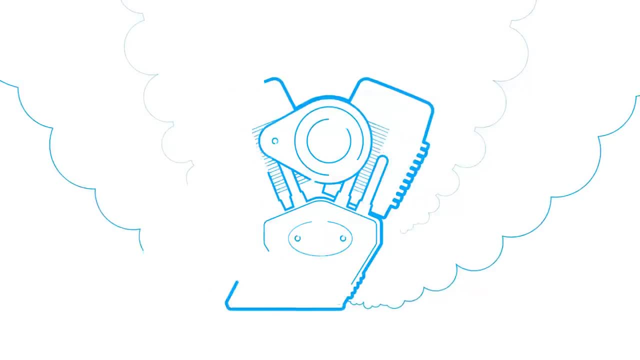 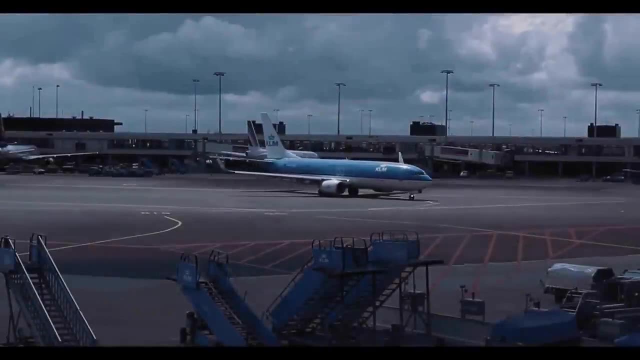 Invisible winds carry planes into the air and make cycling harder. Imagine you could actually see the airflow in all detail. At the Delft wind tunnel facilities, researchers 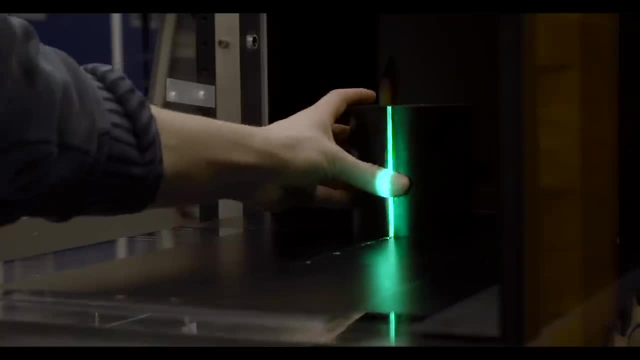 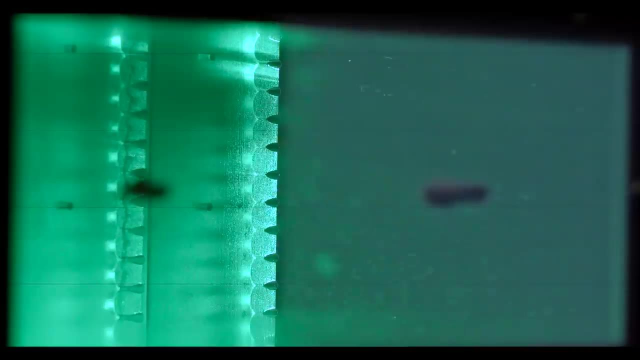 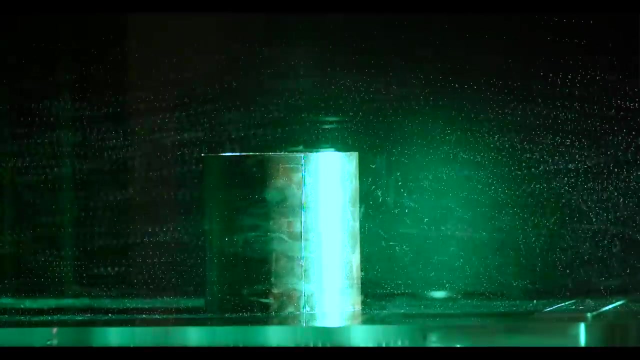 develop a technique that shows air flowing around objects. The objects may vary from simple cylinders to live athletes. The air is made visible by adding micron-sized bubbles containing helium to the flow. These floating particles light up under the beam of a strong laser. This technique is called particle image velocimetry, or PIV. 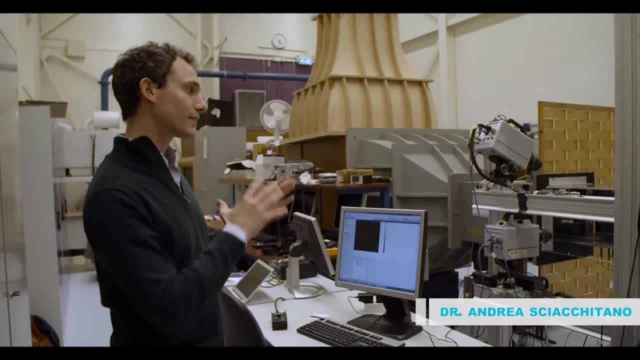 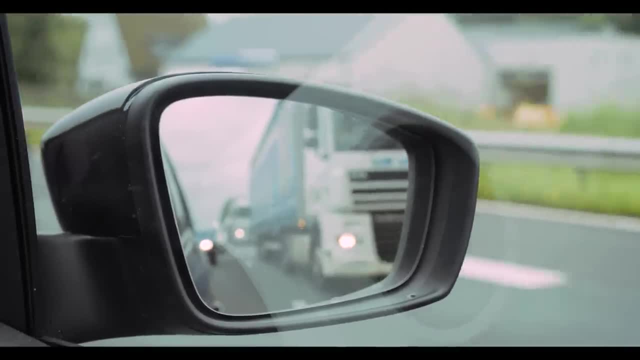 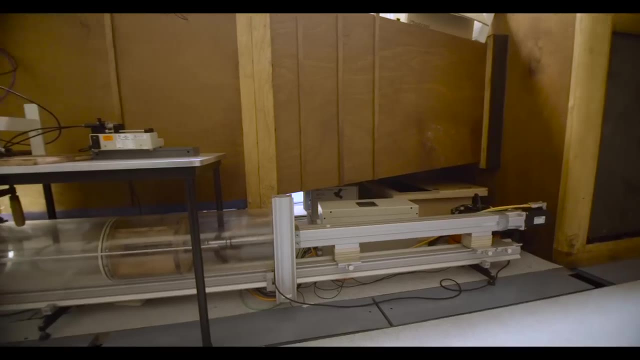 What you saw here is just a cylinder on a flat plate, but you can consider this as a simplified model of a side mirror of a car. So when you're driving your car, the flow goes around the side mirror and there is a phenomenal flow separation and reattachment on the window of the car that causes noise. 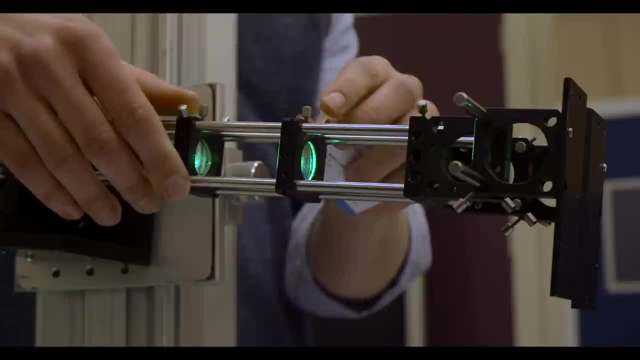 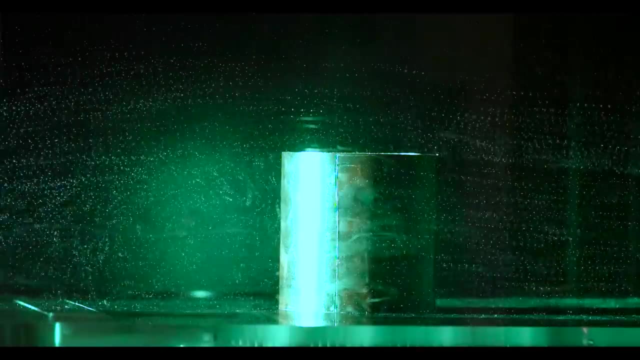 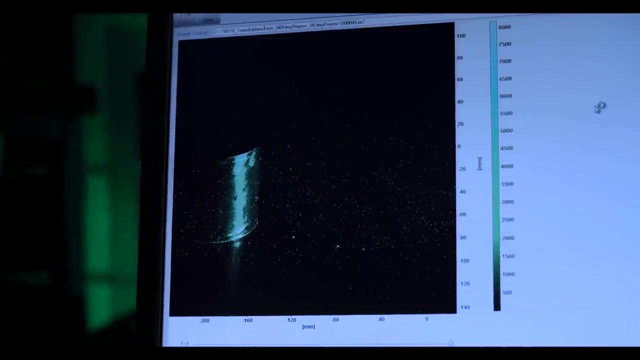 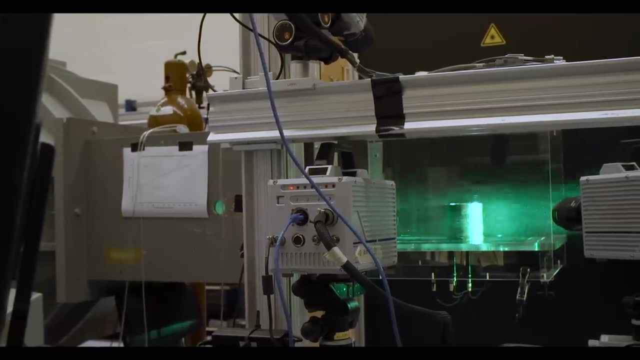 The helium bubbles allow the researchers to work in volumes as big as a beer crate. This is quite a leap forward compared to the iPhone volume they could handle before. Besides noise, this flow separation also causes huge drag forces. Using multiple high-speed cameras and a complicated algorithm, the particles can be evaluated. Car manufacturers can use this PIV technology to improve car aerodynamics and reduce your fuel costs. 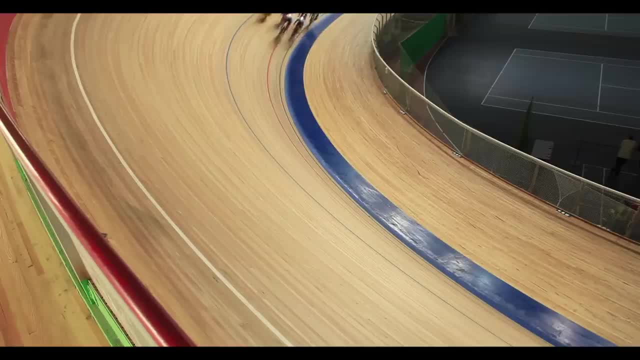 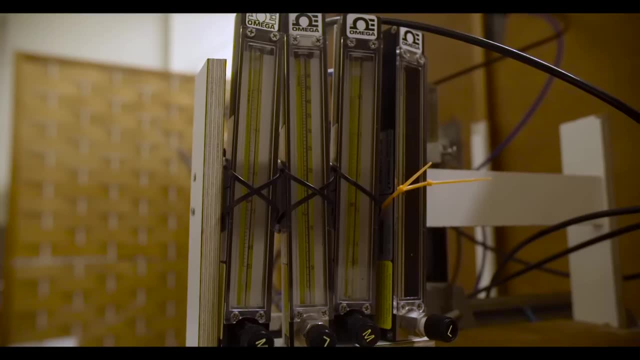 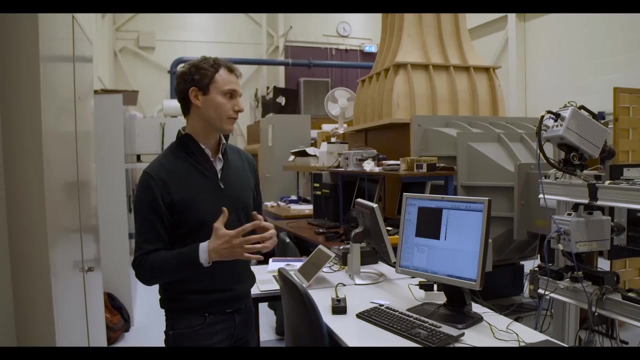 Other interesting applications are in sport aerodynamics. A cyclist or an athlete is training on the track, and we introduce a facility composed by helium-filled bubbles injectors and cameras and lights where the athlete passes through. The advantage, of course, is that we can perform measurements in the track. 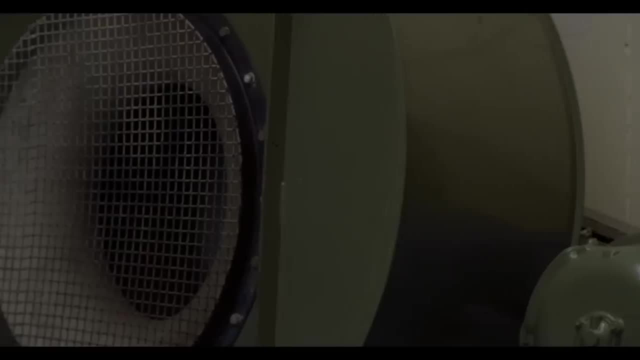 PIV is not only able to reduce your fuel costs and help our athletes go faster, it could also change the way we engineer aerodynamics.